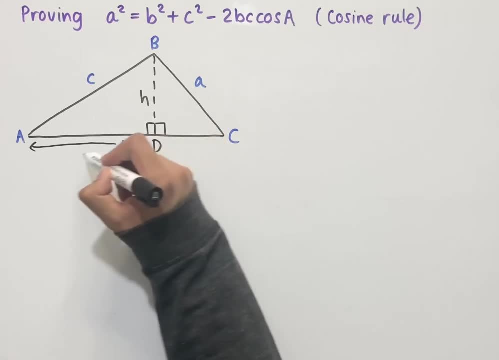 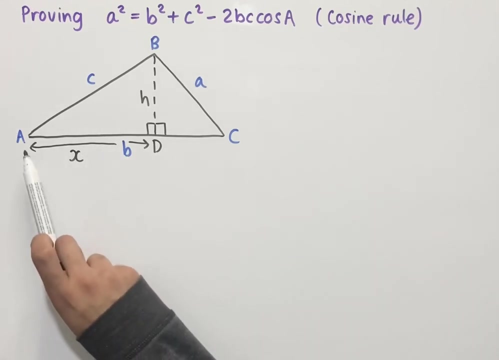 lowercase X. So this full length here we're going to label as lowercase X, and so if the length from A to C is lowercase B, then the length from D to C is going to be that full length minus the length from A to D, In other words as 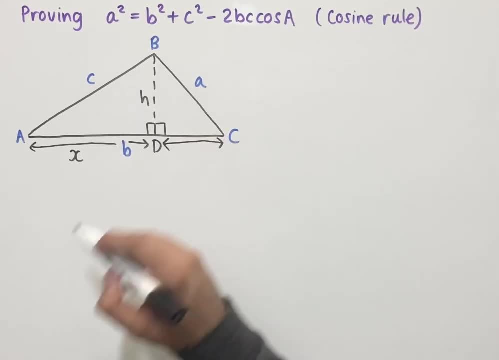 an expression we would have, that D to C is equal to B minus X. Now, looking at the cosine rule, we have a square term for A, we have a square term for B and we have a square term for C. This looks very similar to Pythagoras' theorem and in fact, we use Pythagoras' theorem to obtain squared terms. 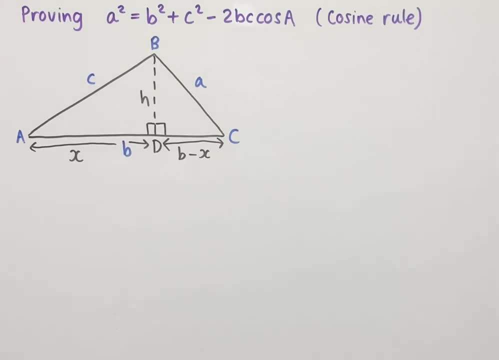 from this triangle and the scenario that we have here, And so the first thing that should come to mind is: how can we get these terms? Well, let's use Pythagoras' theorem, since we have two right angled triangles In triangle B, D, C to start off with. so that's the triangle that's right angled on. 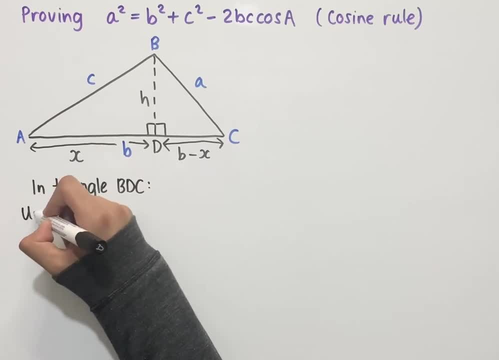 the right. here we have, using Pythagoras' theorem, we get A squared, which is the hypotenuse, which equals to hate squared, which is this side length here of the triangle B D, C, plus B minus X, all squared, Which is the other side length of the triangle B D, C. And now expanding the brackets on the right, 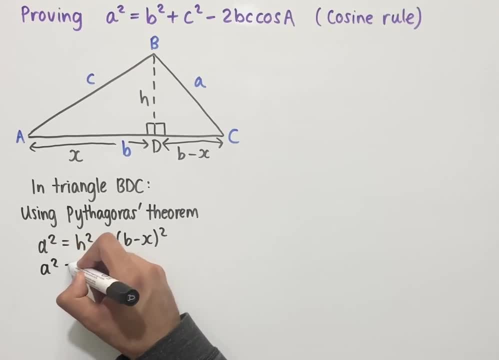 hand side, we get the following equation: So A squared equals to hate squared. Now, if we expand this, we get plus B squared, minus 2BX plus X squared. You might want to take a moment to convince yourself that B minus X, all squared, leads us to these three. 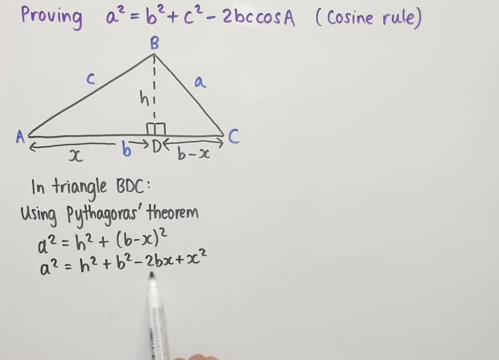 And so we begin to see that this expression is starting to look quite similar to the cosine rule that we have here. There are a few terms that are slightly different, such as hate squared, X squared and the X within minus 2 BX. However, we have some similar parts, such as A squared and B squared. We also apply 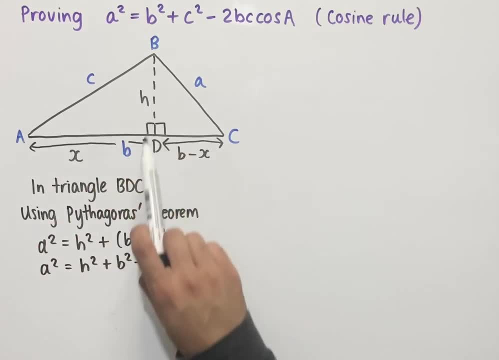 Pythagoras' theorem in triangle ABD. then we get the following equation: So we have the hypotenuse squared, which is c, squared which equals to the base of this triangle ABD, which is X, and we square that plus the other side length or the. 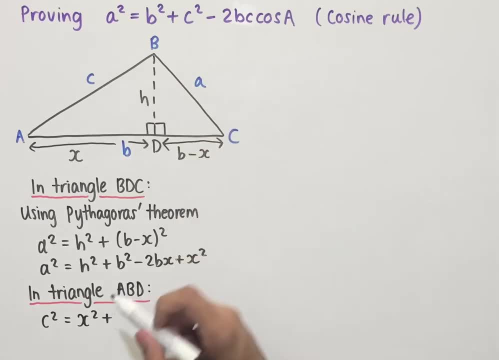 perpendicular height of this triangle, which is H, and so we square that, and so we see that both this first equation that starred here and this second equation that starred here both have H squared in common. if we rearrange this equation here for H squared, in other words make H squared the subject, then 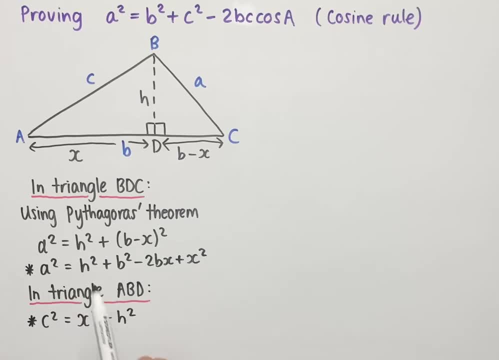 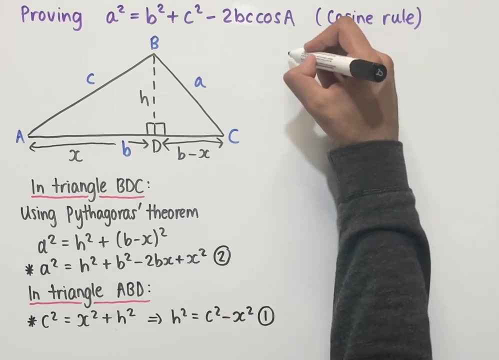 substitute that into this equation, we can get rid of the H squared and further get closer to proving the cosine rule. here we end up with: H squared equals to C squared minus X squared. we label this equation as equation two: 1 and we label this equation as equation 2, then the next step involves substituting equation 1. 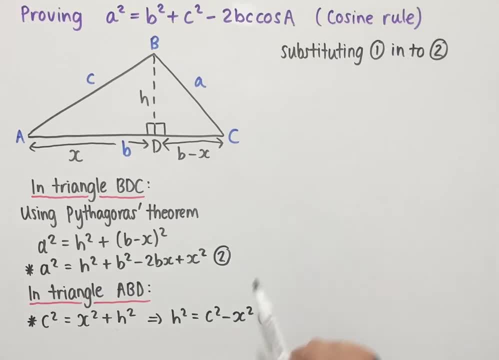 into equation 2.. So this would result in the following: So, looking at equation 2, we have a squared which equals 2 and now, instead of writing hate squared, we're going to write c squared minus x squared, since we're substituting equation 1 into equation 2.. So we have c squared. 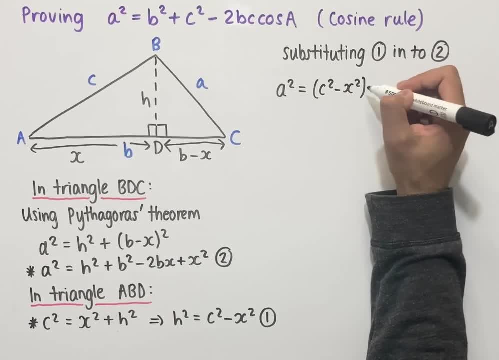 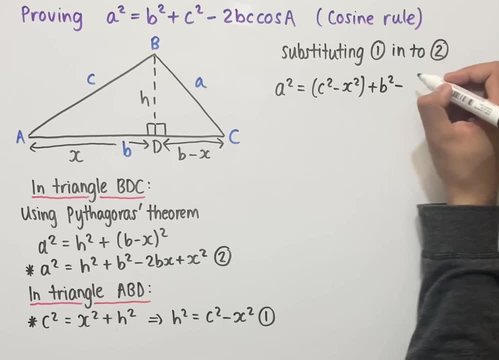 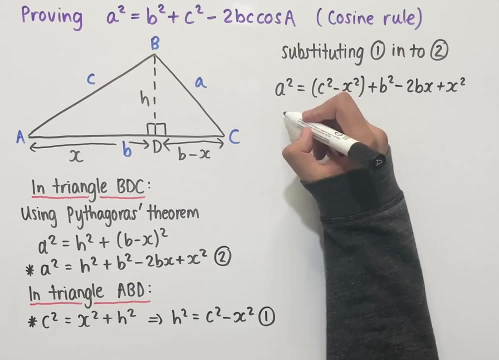 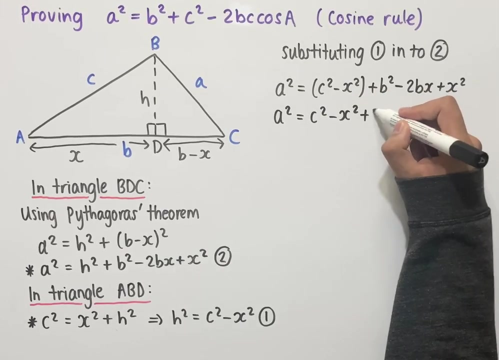 minus x squared, which is our substitution, and so we've written that in brackets: plus b squared minus 2bx plus x squared. So in this case the brackets don't make a difference, so we can get rid of those, and so we have a squared equals to c squared minus x squared plus b squared minus. 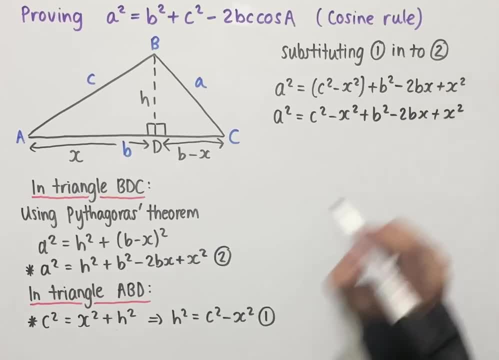 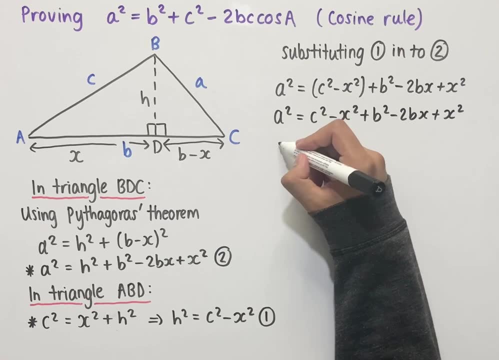 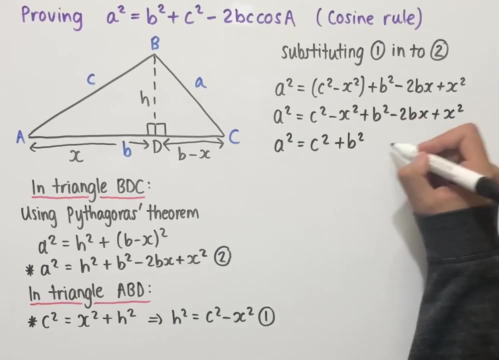 2bx plus x squared. And now we're going to write a squared which equals 2bx plus x squared. Now we see that minus x squared and plus x squared cancel, and so we're left with a squared equals to c squared plus b squared minus 2bx. So again, comparing what we have so far with, 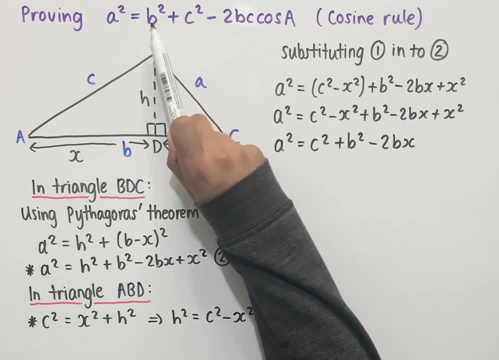 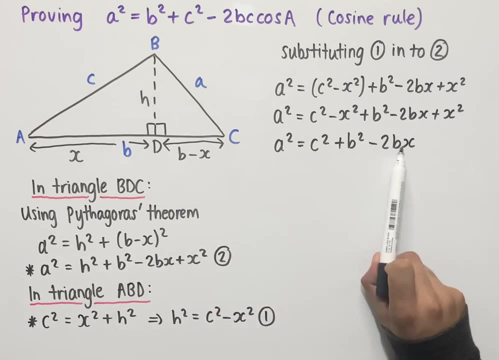 the cosine rule. we see that we've got a squared, we've got b squared, we've got c squared and we've almost got minus 2bc cos a. Instead, we've got minus 2bc cos a. Let's rearrange this so that the terms are in order of the cosine rule. So we have a squared. 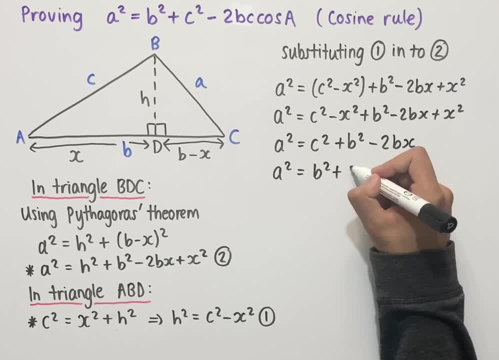 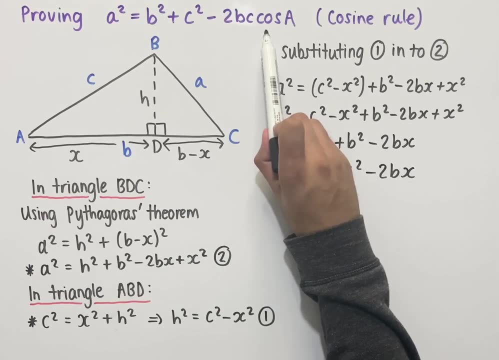 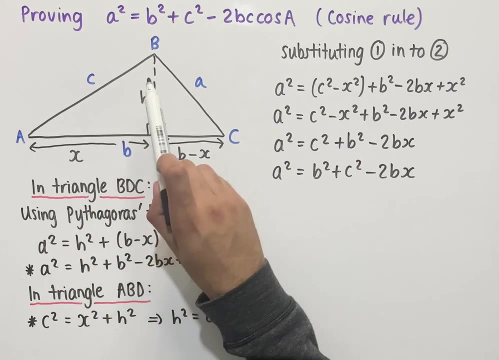 equals to b squared plus c squared minus 2bx. Instead of having x, we need c multiplied by cos a, And so, since we have cos a, we see that in this triangle we have a right-angled triangle on the left where the vertex here is labeled a, And so we can work out the cosine rule. 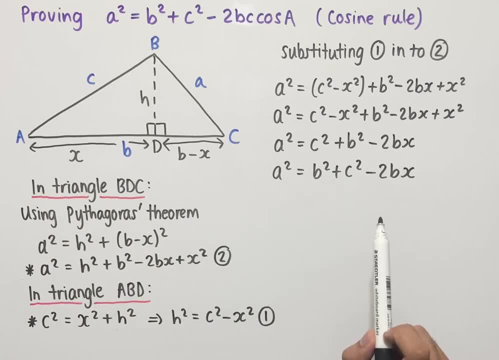 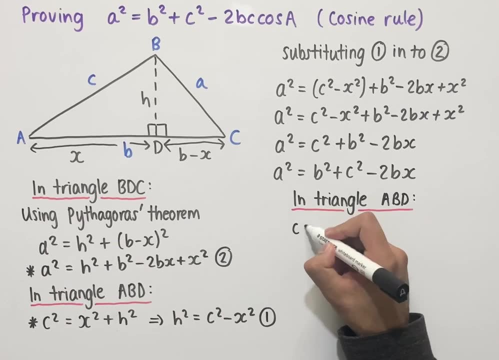 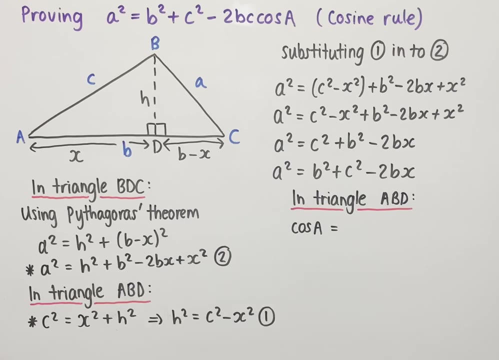 We can work out cos a to obtain an expression for x which we can then substitute in. So in triangle ABD we have cos a equals to. So whenever we take cos of an angle, we look at the adjacent side over the hypotenuse And we can only use trigonometry or SOHCAHTOA. 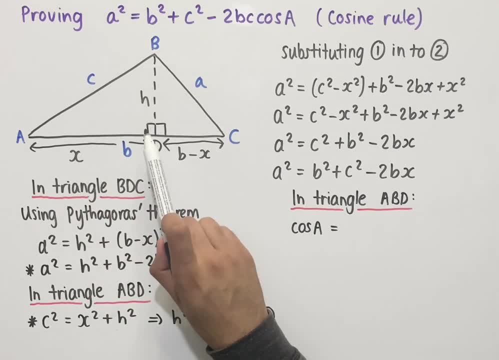 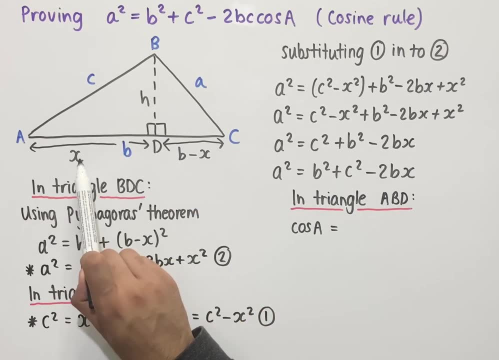 when we have right-angled triangles. Since we have a right-angled triangle here for ABD, we can use this, So cos a is equal to the side, the adjacent side is labeled as X. over the hypotenuse, the hypotenuse in. 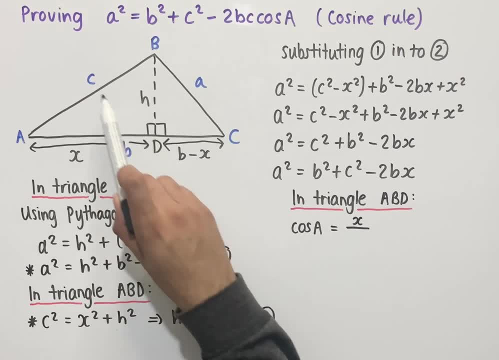 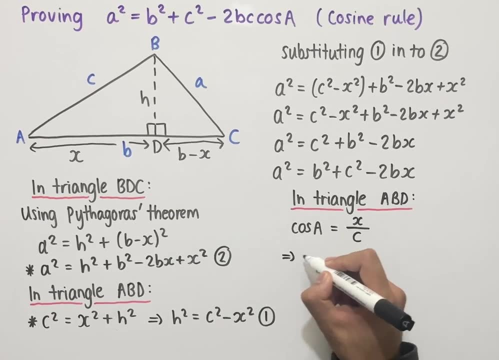 this case is the side that's opposite, the right angle, and so that would be C. so we have cos A equals to X over C. multiply both sides by C, we end up with C multiplied by cos A, which equals to X. so finally, if we substitute C cos A, 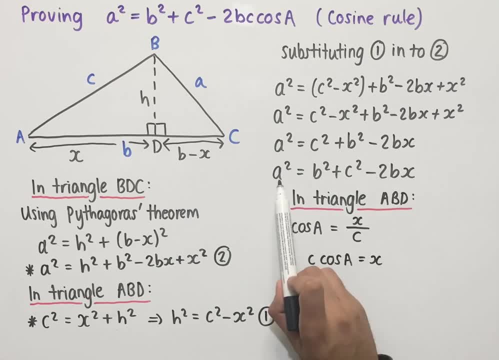 equals to X into this equation. here A squared equals B squared plus C squared minus 2 B, X. we get that A squared equals to B squared plus C squared minus 2 B, and instead of writing X, we're now going to write C cos A, and we see that this 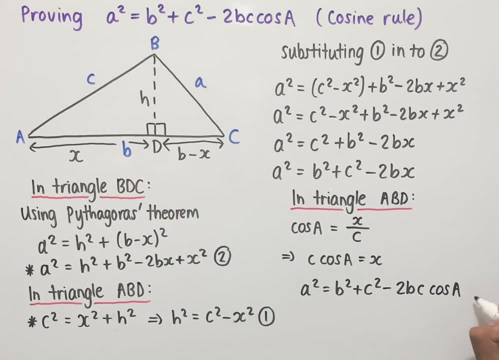 indeed is the cosine rule here, so we've proved the cosine rule.